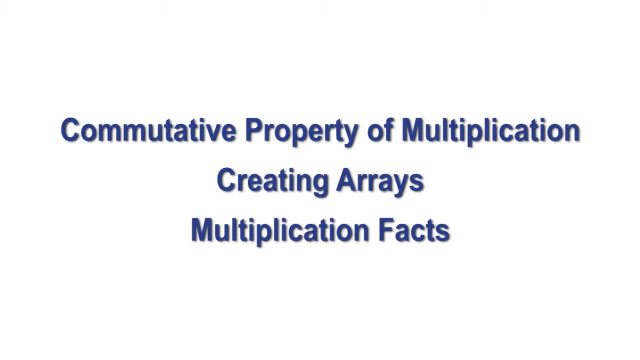 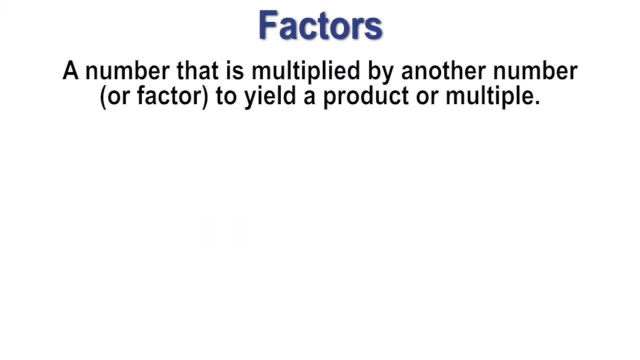 to aid in the learning process. Let's move on to the new skills and concepts for this chapter. The first concept students will learn is factors. A factor is a number that can be multiplied by other numbers to get a product. In this chapter, students will be required to list factors for a given number. 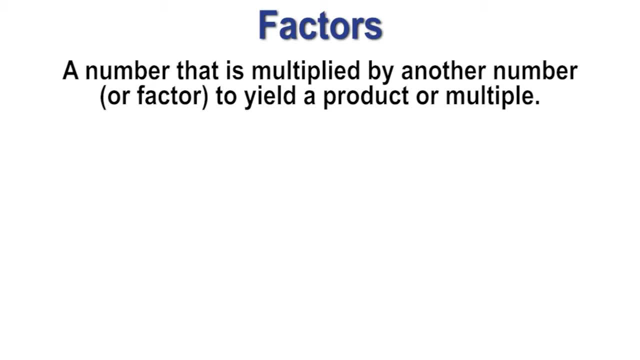 between 1 and 100.. Students will learn multiple ways to find factors. Let's list the factors for 12.. Every number has a factor of 1 and itself. so the first factor pair is 1 and 12, because 1 times 12 equals 12.. These factors can be modeled using: 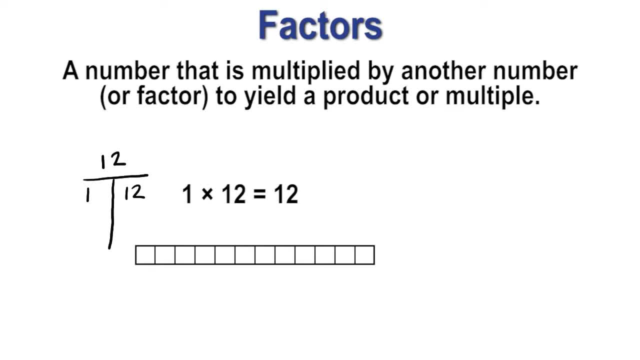 an area model with one row of 12 or they can be listed in a T-chart. The factors 1 and 12 can be switched to 12 times 1 and still result in the same multiple of 12.. As an area model, this will be 12 and 12.. 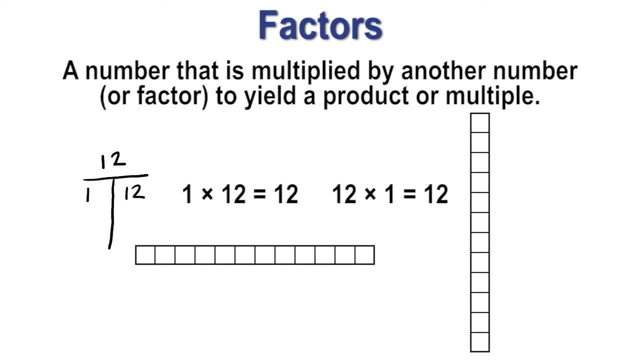 rows of 1, but again resulting in the same product of 12 and the same factors of 1 and 12.. The next factor to consider would be 2.. 2 times 6 is 12, so 2 and 6 are another factor pair for 12.. This can be modeled with an area model of 2 rows. 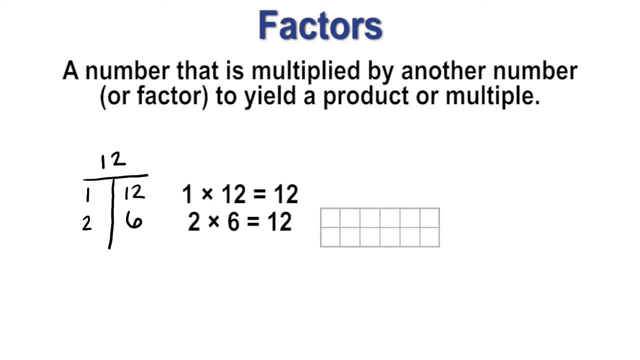 of 6 or listed in the t-chart. The last factor pair is 3 times 4, as modeled with the area models and the t-chart. The next concept students will learn is multiples. A multiple of a number is the product of that number and any other. 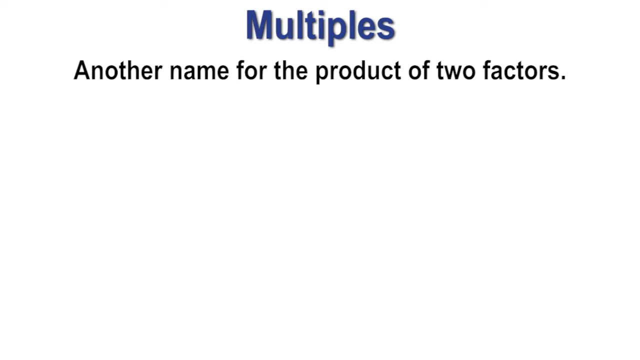 whole number. Students will be taught a wide variety of strategies to find multiples and determine if a number is a multiple. Let's find the multiples of 6 up to 100.. One way would be to create sets with 6 in each set, starting with. 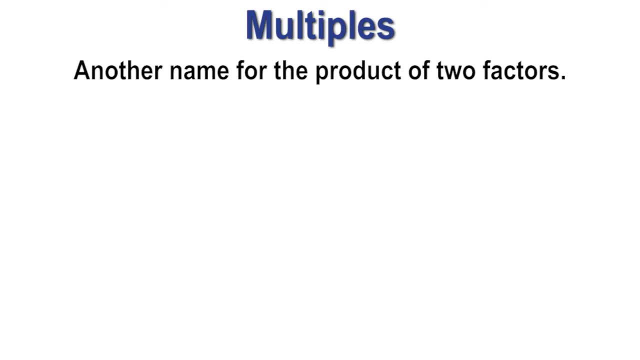 0. There would be nothing, and as an equation this is written as 0.. 0 times 6 equals 0.. The next set would be one set of 6, or 1 times 6 equals 6.. The product 6 is a multiple of 6.. This can also be shown on a number line as 1. 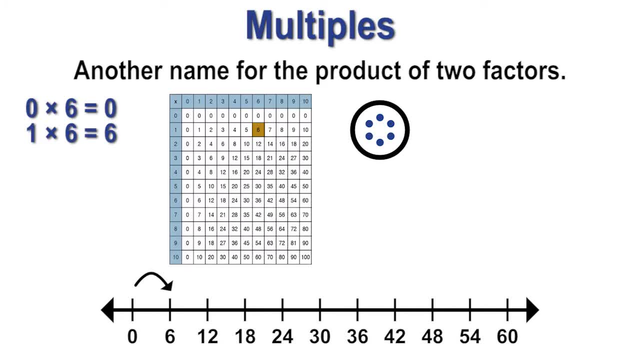 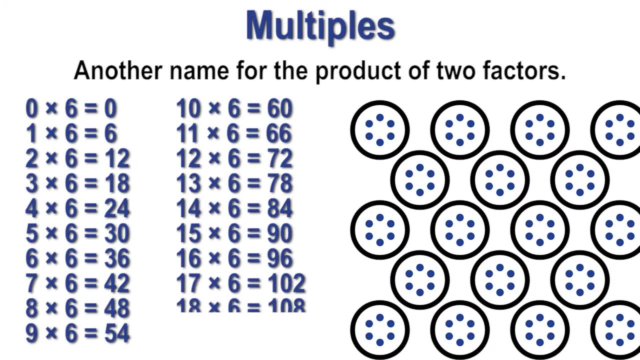 jump of 6, or on a multiplication chart as 1 times 6.. This will go on forever as long as the multiplication equation created has one factor of 6.. Students will then apply this knowledge to determining if a given number is a multiple of a given factor. For example, is 18 a? 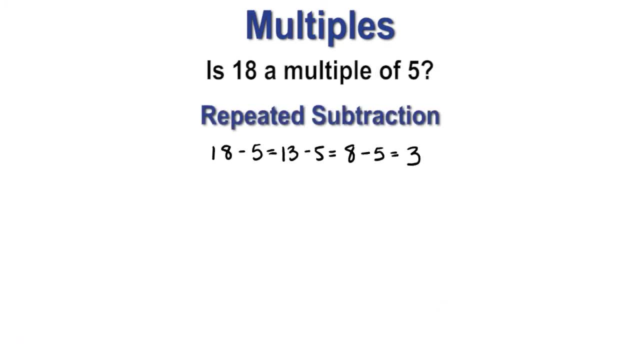 multiple of 5?. Students can use their knowledge of repeated subtraction or they can divide 18 divided by 5, to see that 18 is not a multiple of 5.. Students may also skip count by 5's to realize that the pattern goes from 15 to 20 and 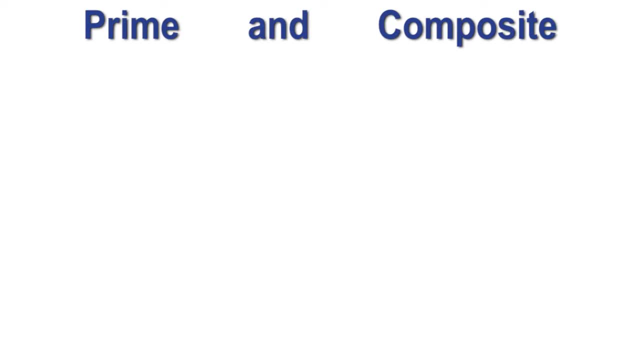 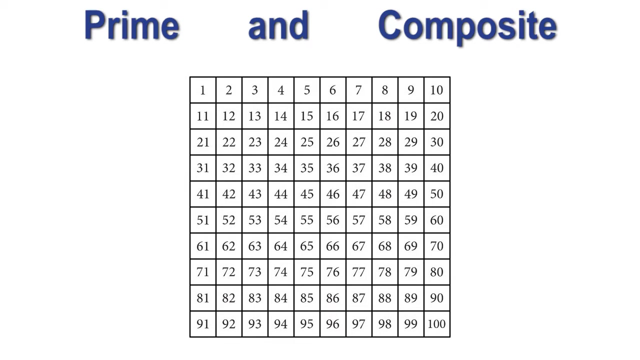 18 is not included. The next concept students will learn are prime and composite numbers. Any prime number has exactly one pair of factors, one and itself. All other numbers are composite numbers. Students will use a hundreds chart to explore all the prime numbers to 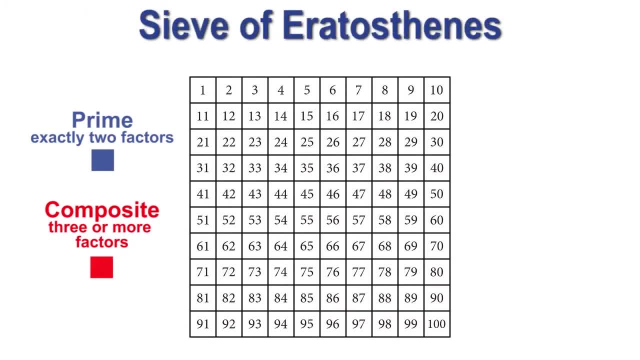 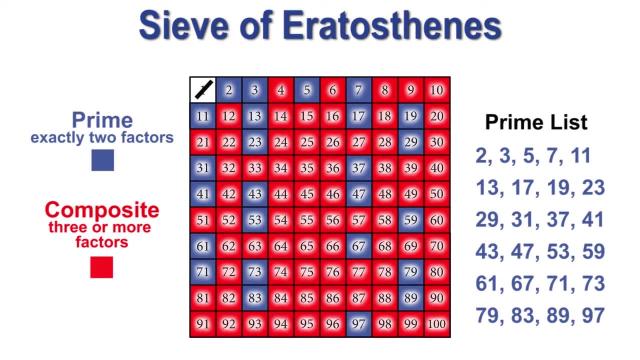 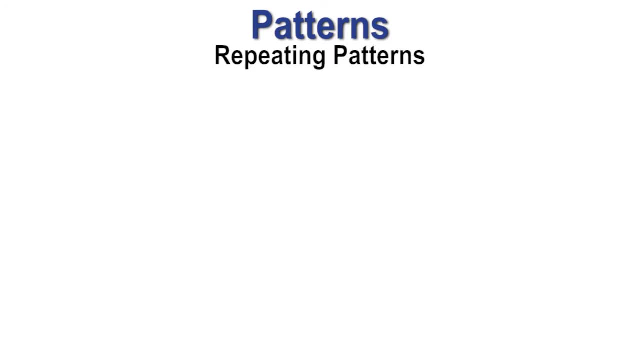 100, also referred to as the sieve of Eratosthenes. They will shade all prime numbers with one color and all composite numbers with another color. Finally, students will now explore patterns with known rules. Students will start by examining repeating patterns, which are patterns that have a core. 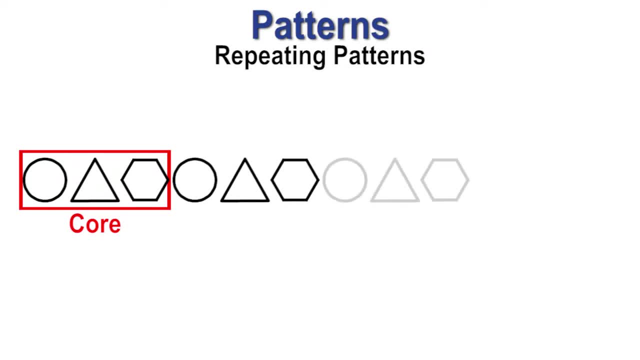 made up of a set number of terms and that are repeated over and over again. The word term refers to one of the ordered pieces in the pattern. This pattern has a core pattern of circle triangle hexagon. This can be thought of as an ABC pattern. Term A is a. 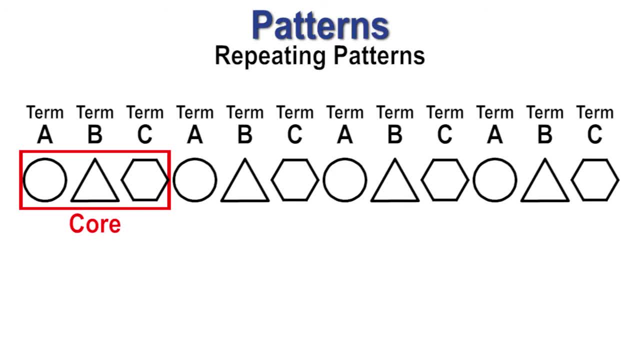 circle. term B is a triangle and term C is a hexagon. Students will then examine the relationship between the term number and the corresponding shape. Every multiple of three is a hexagon. What would the 16th term in the pattern be, without actually continuing? 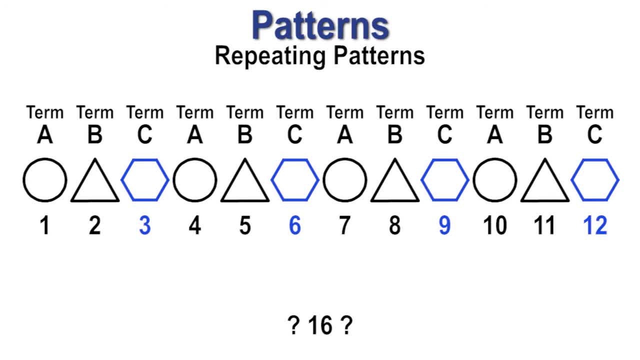 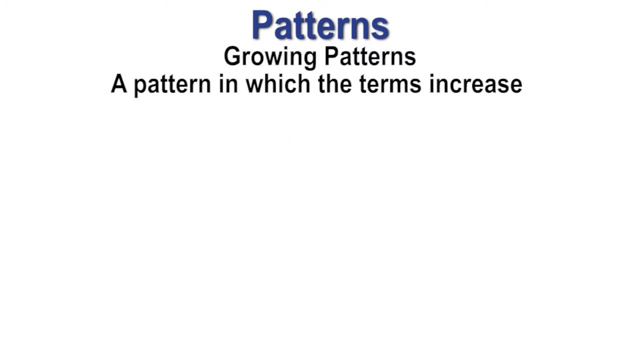 the pattern to 16?? Well, if every multiple of three is a hexagon and 15 is a multiple of three, then 16 would be one term after the hexagon, which is a circle. The other type of pattern students will learn are growing patterns, which are patterns where the value 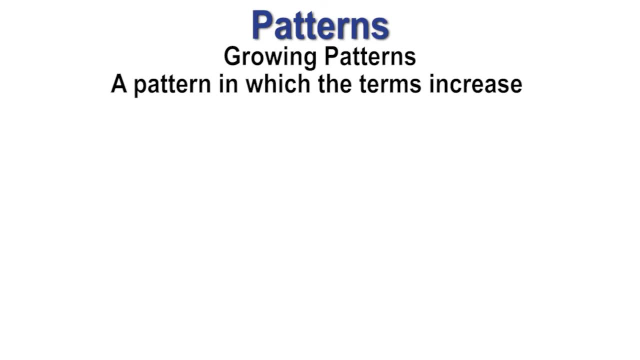 of the terms increase each term. This will be a lesson where students will focus on discussion and discovery, because students see how patterns grow in many different ways. Let's examine a growing pattern. The rule is: multiply by 2, start on 2.. The first term will be 2.. The 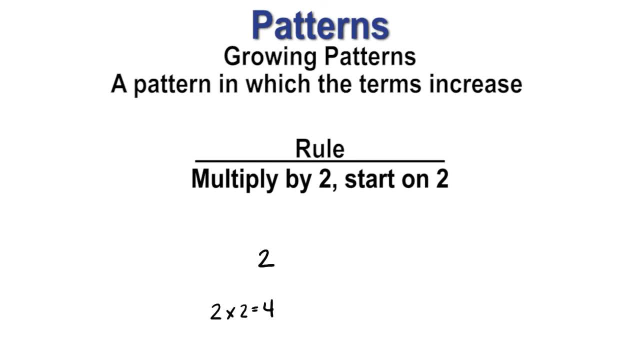 next term will multiply the previous term by 2,, so 2 times 2 is 4.. The third term will multiply the previous term- 4, by 2, for an answer of 8.. The objective for this chapter was to focus on 2..